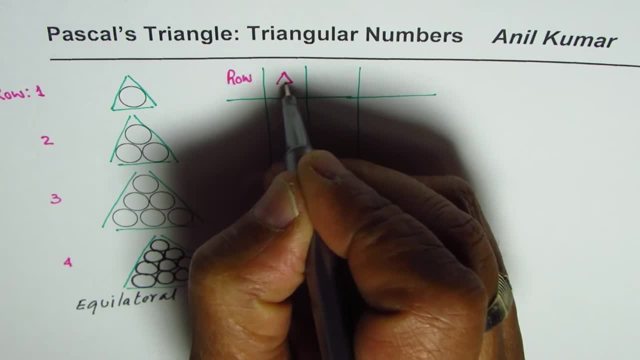 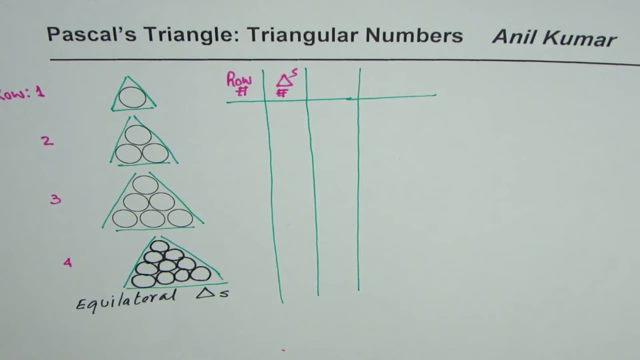 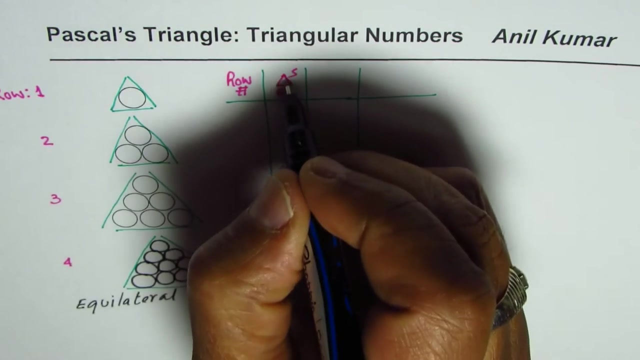 rows and here we'll write the number of triangles. okay, so row number and triangles number. to begin with, in the very first row we have only- i mean i should have written circles, so we'll write circles in the triangle. so in row one we have one circle. 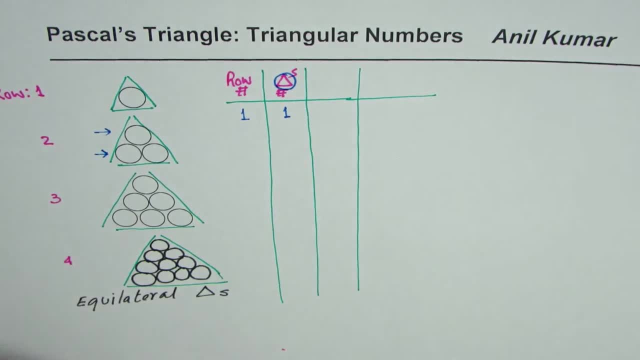 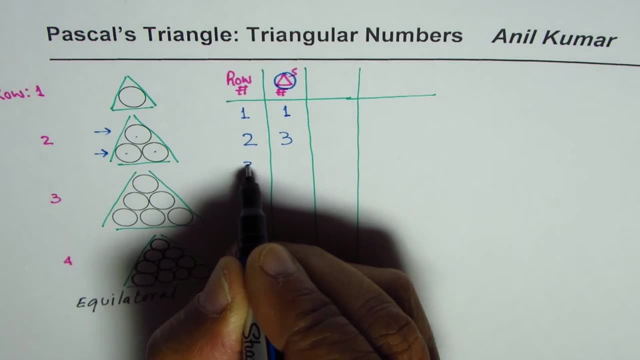 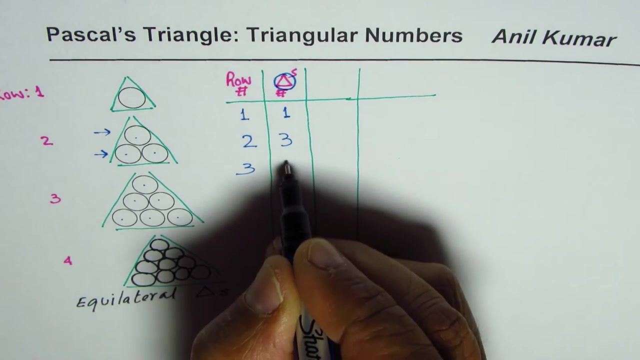 if we have two rows. so these are the rows which we are talking about. in two rows we have three circles. these are the three circles we're talking about. third row has three and third row three more, so you add three to it. you get six. fourth row in addition to whatever we had. 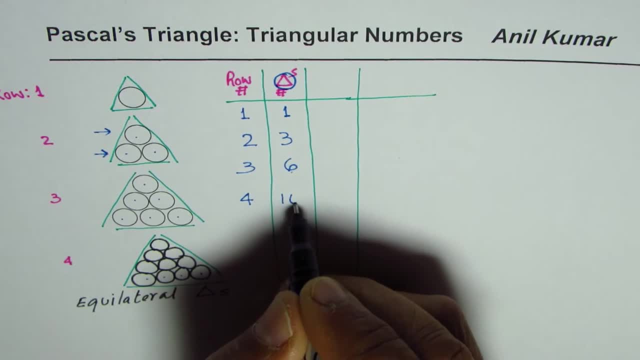 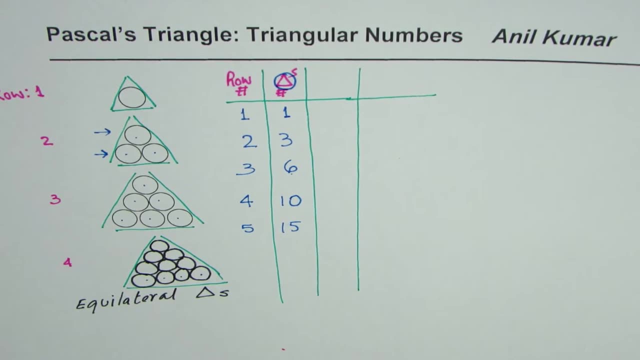 it has four more six plus four is 10. with that pattern, fifth will have five more 15, and so on. right, so that is how the pattern is going to increase. so what we see here is a pattern where, with every row, the number of circles increasing- in our case, is same as the row number being. 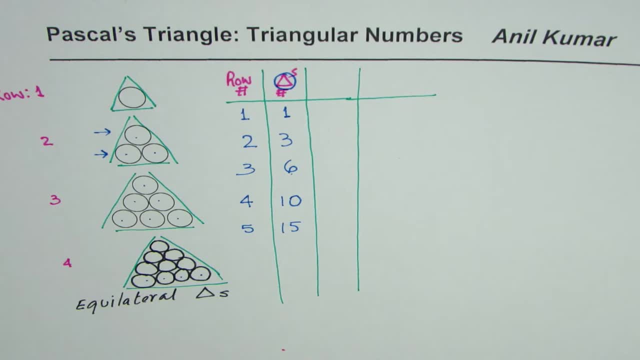 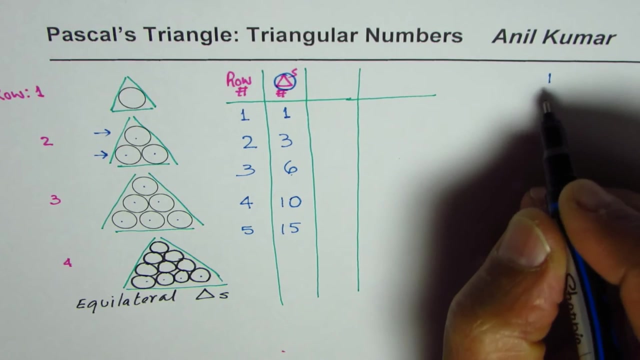 increased, correct? that is the pattern which we notice now. is there a relation of this pattern with pascal's triangle? that is the main idea. so let us see if there is one. so let's start with row zero for pascal's triangle, and then, when you 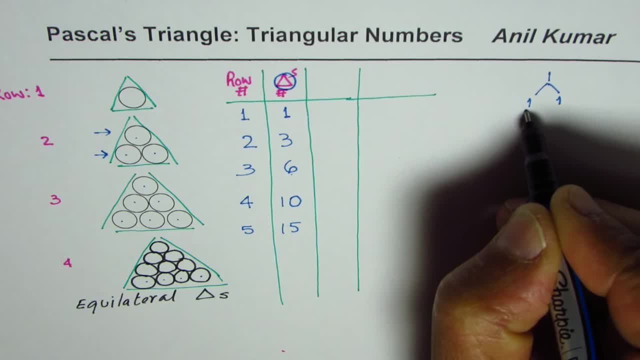 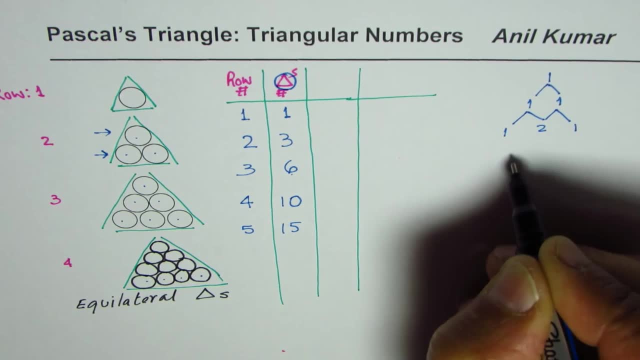 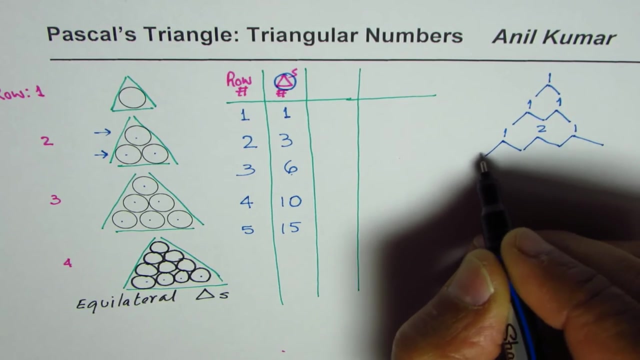 expand. in row one we have these two ones, and in the second row we have three terms, so one, two and one, and in the third row we have four terms right, so with every row there are four numbers right. so when you add one, one plus two is three. 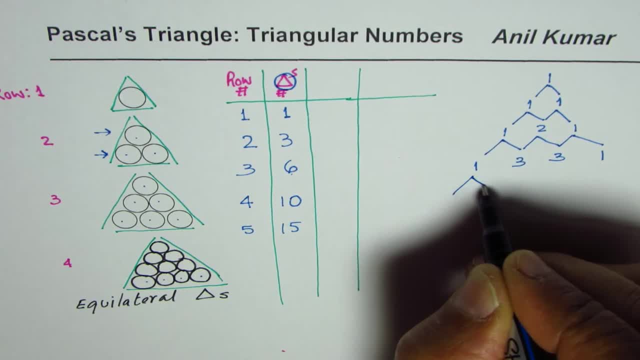 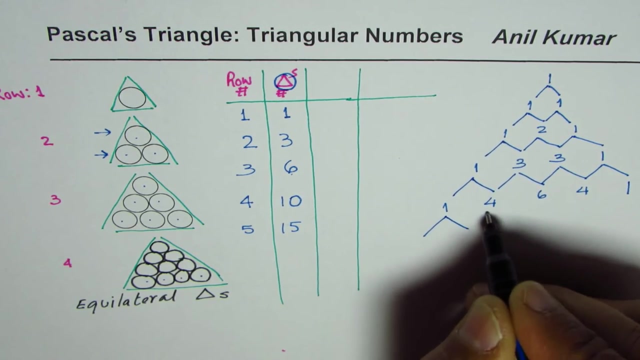 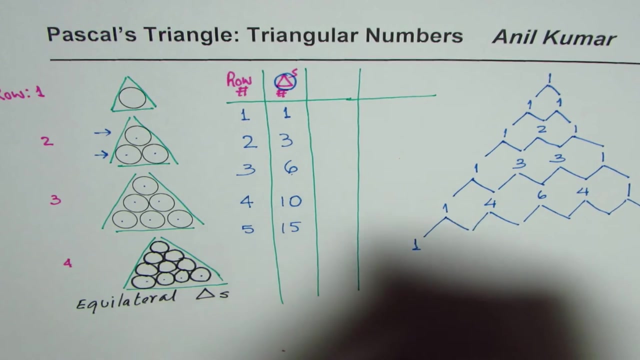 three and one, and in the next row we have one more term, right? so so that is it. so we have one three plus one, four, three, three, six, four and one. and if we increase this? so what happens? so if we increase this, uh, it is something like this, and then we'll compare with our numbers. 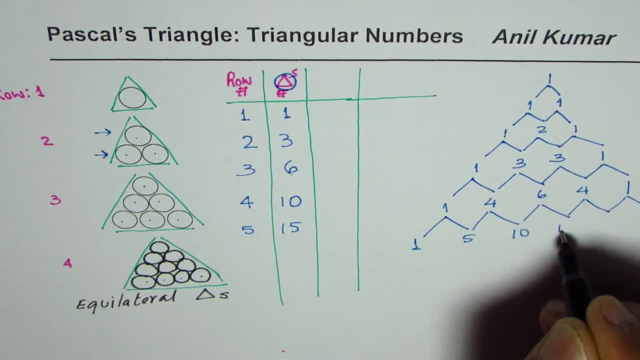 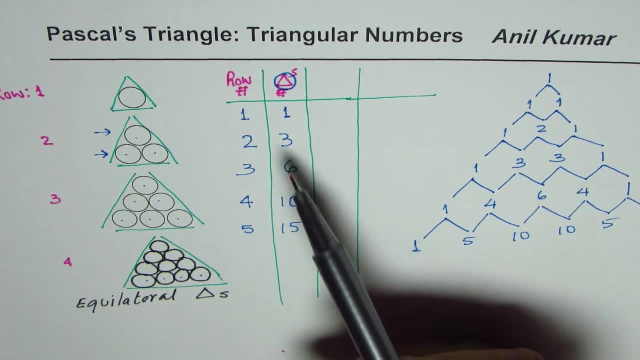 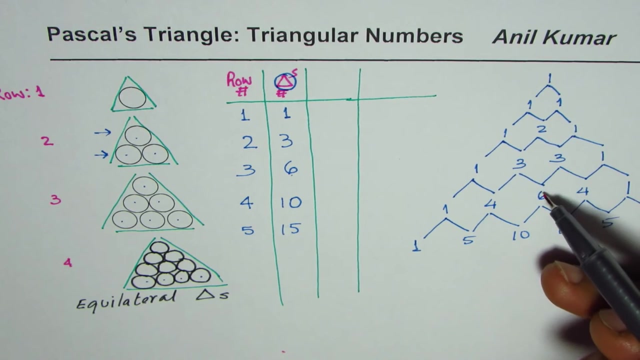 four plus one, five, six plus four, ten, six plus four, ten, then 5 and 1. now what we are getting here is numbers like 1, 3, 6, 10 and 5. let's see these diagonals: 1, 3, 6, 10 and 15, right. so so if you notice this, 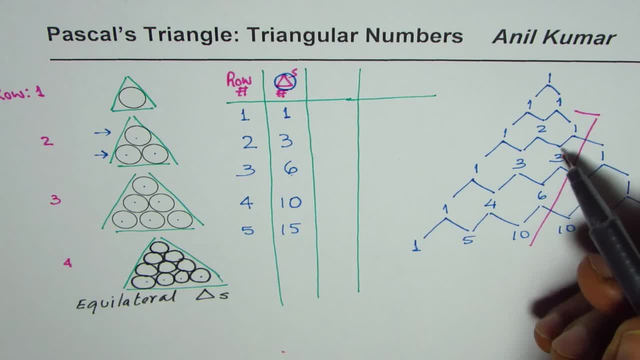 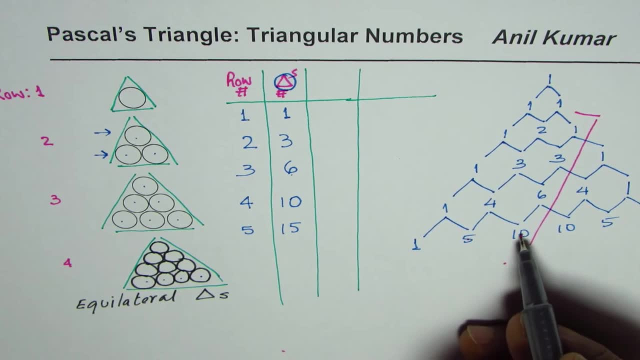 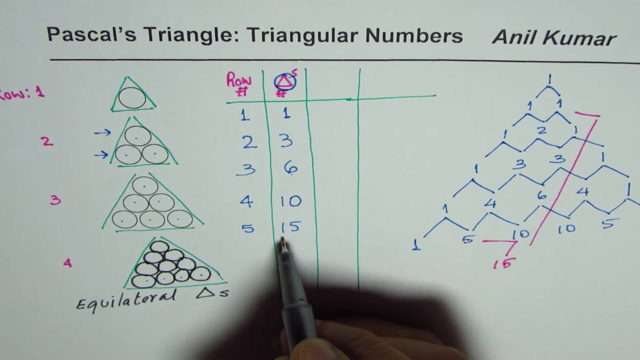 particular diagonal, which is the third diagonal: 1, 3, 6, 10 and if I expand this, the number here will be: when you add 5 and 10. do you see that when you add 5 and 10, you'll get this number correct, which will be 15, right? so so we get the. 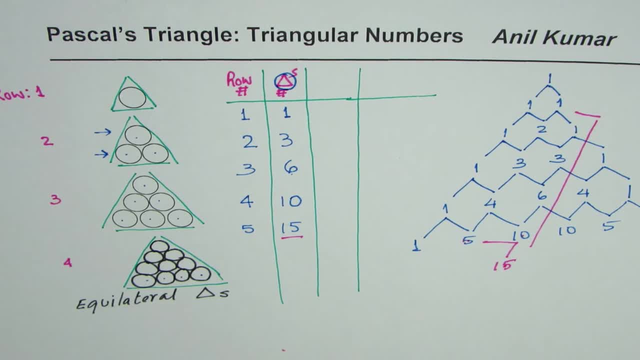 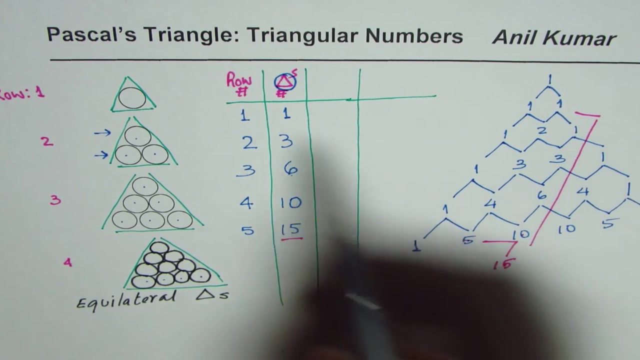 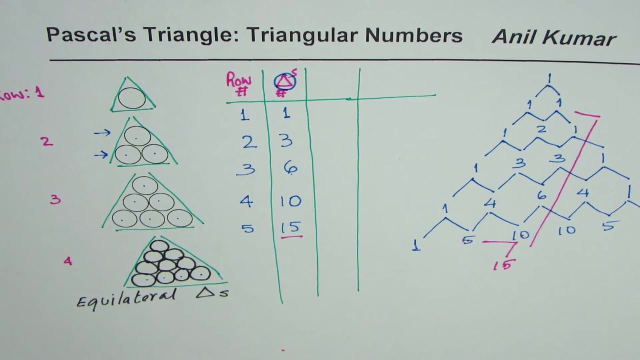 next number. so what do you notice here is that these numbers here correspond to the terms within the Pascal's triangle, right? so so the position here we can write for each. so the position here we can write for each, the position as in this particular case. let me write this as in terms of the 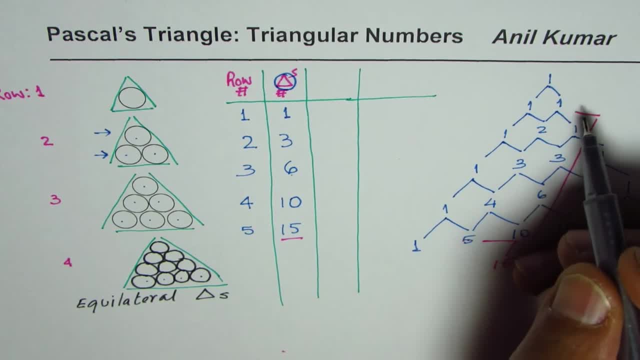 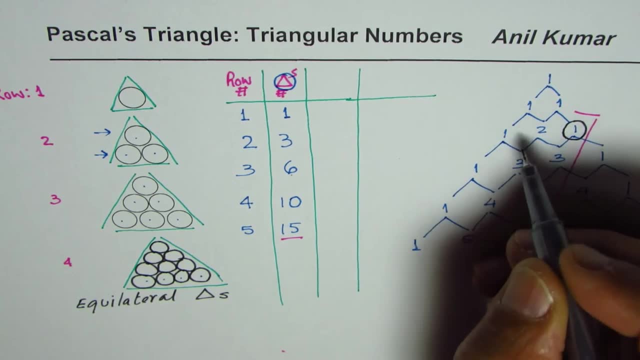 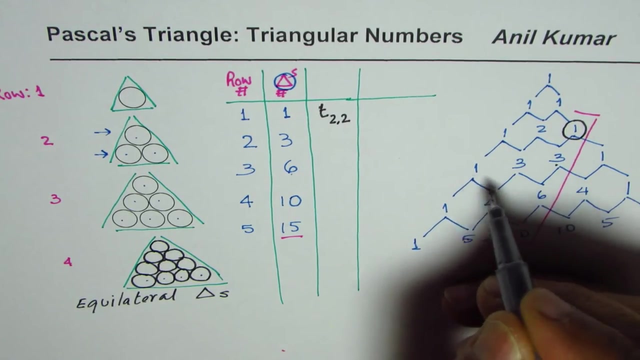 term number using Pascal's notation. so here we are saying: this number right, so it is row number is 2 for us, correct, and 0, 1, 2, so it is T 2, 2, right. this position is row number 3 for us: 0, 1, 2, 3, so it is T 3. 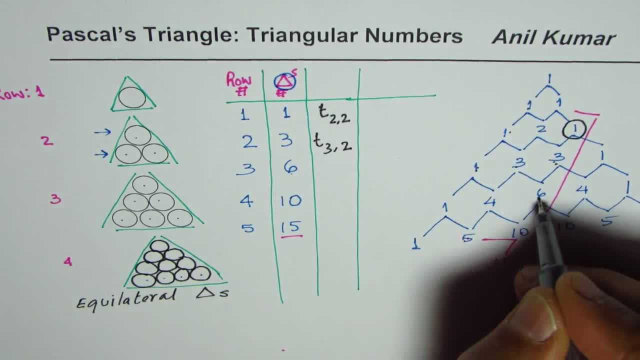 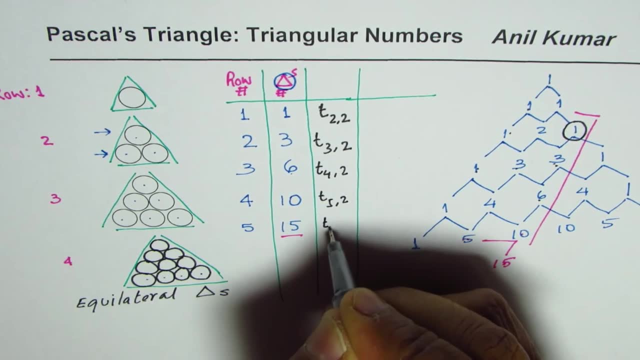 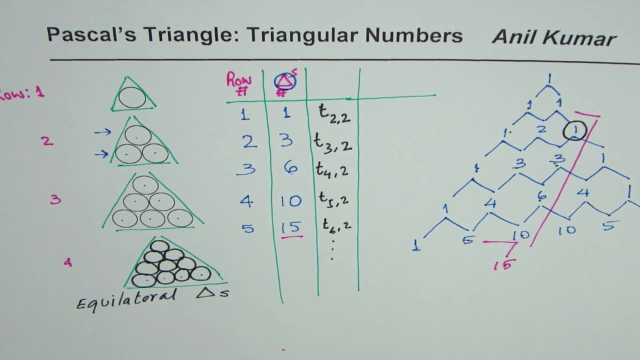 0, 1, 2, T, 3, 2. similarly, the other positions are T 4, 2, T 5 2, T 6, 2 and so on. so when you relate them, what relation do you see if I have nth row in that? 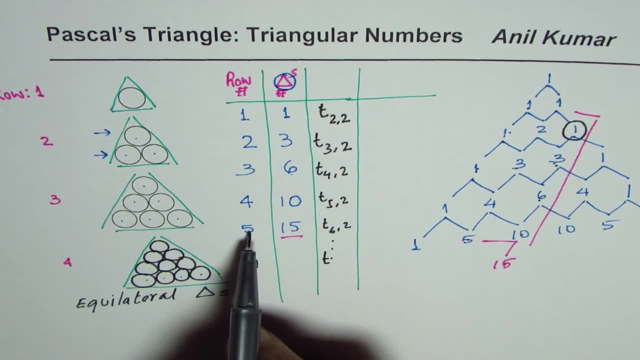 case this should be T. 6 is 1 more than 5, 5 is 1 more than 4, so we have n plus 1- 2. so that is how we can find number of circles in nth row. do you get the idea right? so so if I have 10th row, for example, and if I make this pattern, then 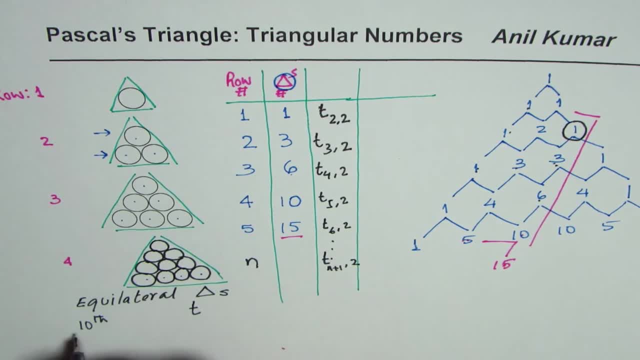 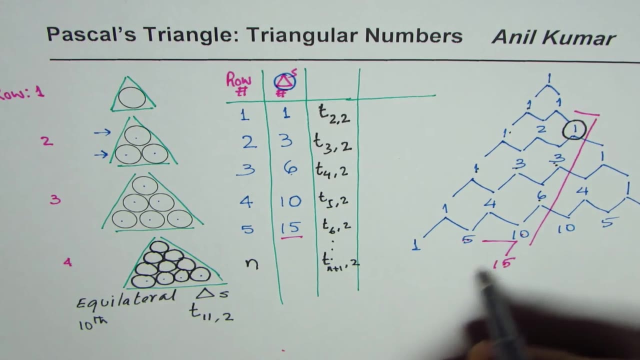 the number of circles will be how many? T? 10 plus 1, 11, 2. do you see that? so we can expand and get the result? now there is another quick way of finding this answer: to find the 11th row, we have to kind of continue with this pattern, as you will. 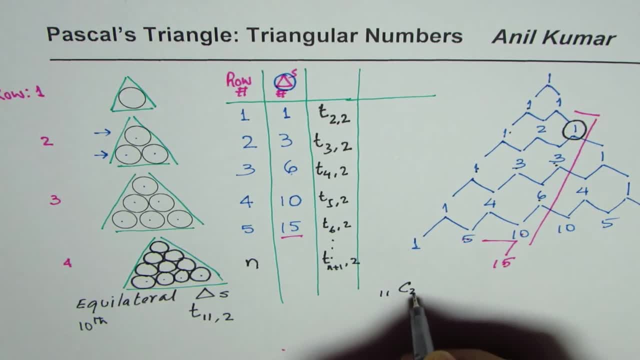 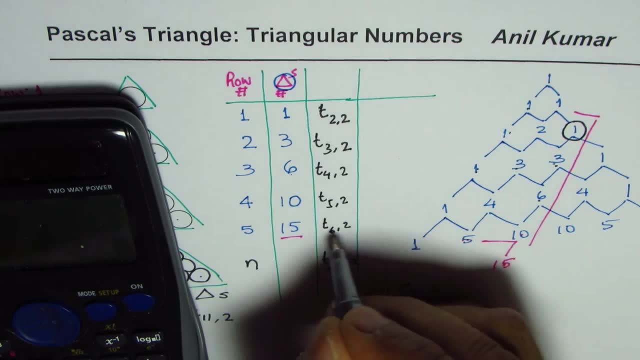 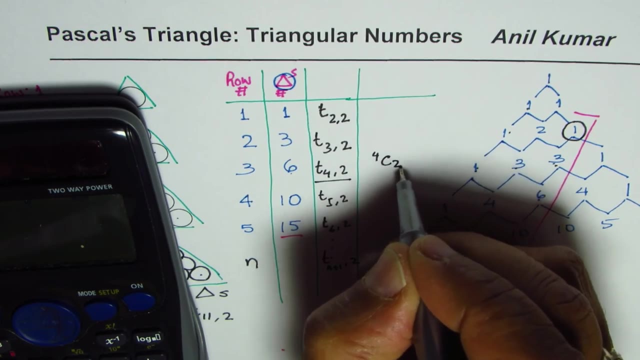 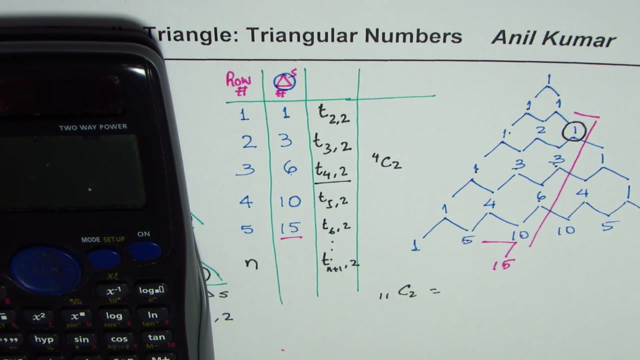 learn. we can use combination 11, C 2 will also give us the same number. let me try it out with the calculator. let me first do check one of these values. let us say we check this, that is 4 C 2. so if I use calculator we say 4, here's a combination C 2. it gives us a number 6. 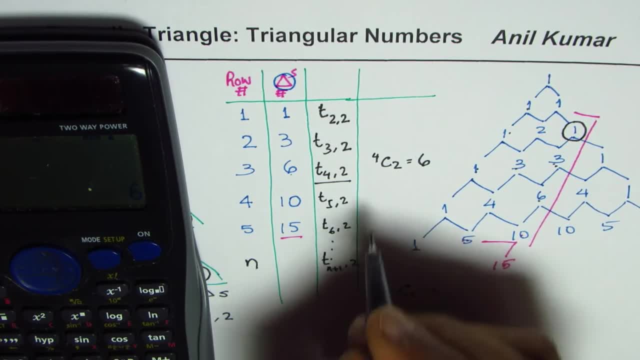 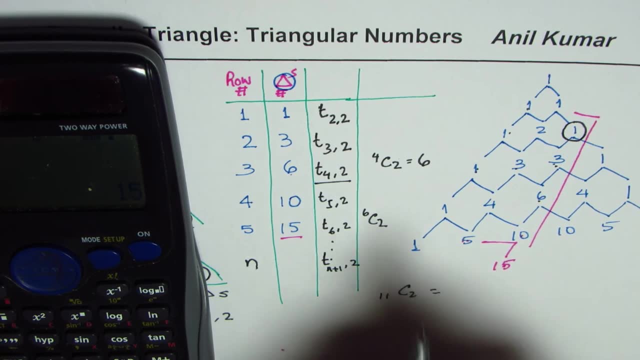 we know it is 6, correct. if I try 6 C 2, so it is 6 C 2, what do I get? I get 15, right, so this is 15 and therefore I could try 11 C 2 also. 11 C 2 will give us. 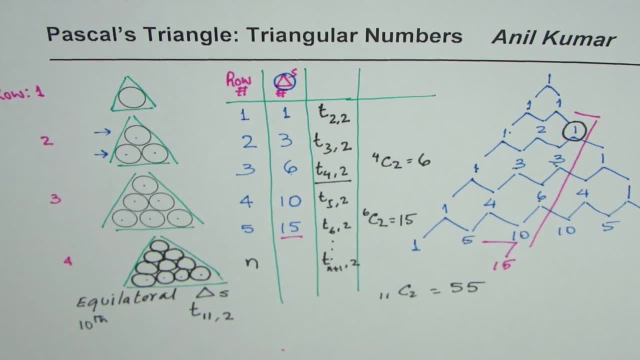 5. so the number of circles in the 10th row. I mean I should say in a triangle formed using 10 rows. so I should not say 10th row, I should rate, say row 10. right, 10 rows will be so many. so let me write down here: we say number of circles in 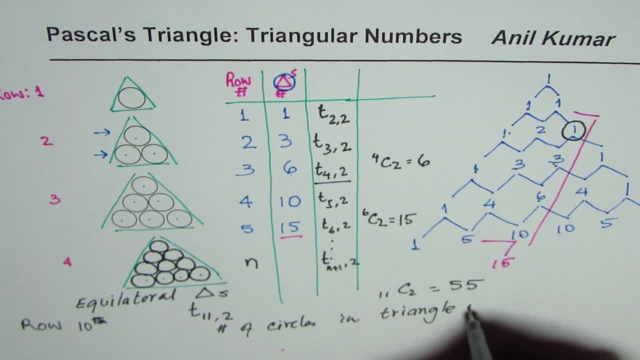 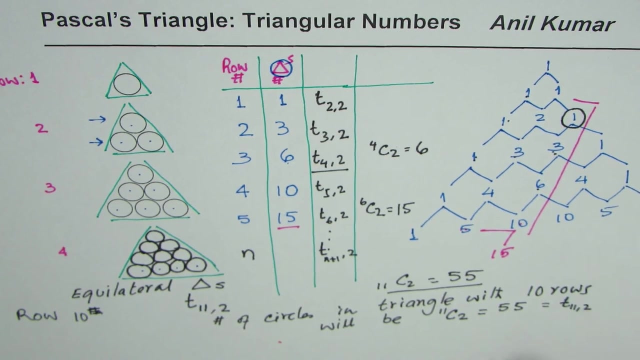 triangle, 10 rows- right? that is absolutely clear- will be 55, will be 11 C 2, 1 plus 10, which is equals to 55, and in Pascal's triangle terms it will be. it will be same as equals to T 11: 2, right? so that is how you can find. 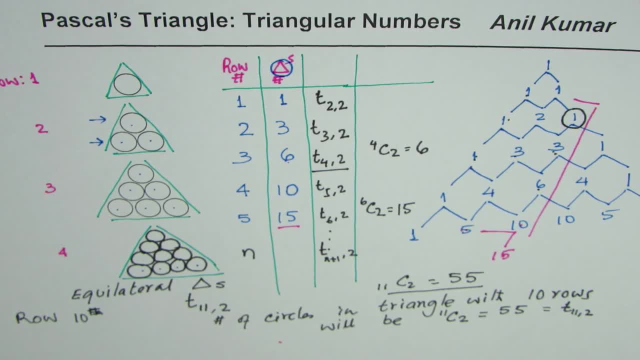 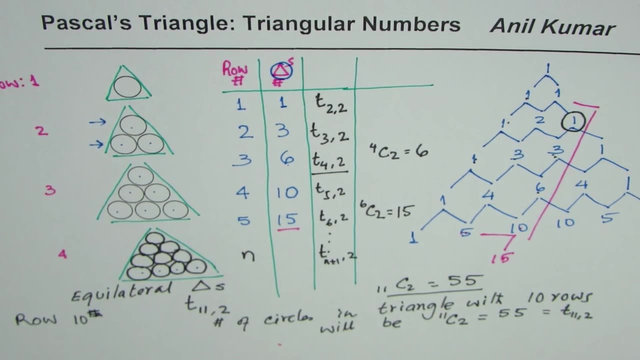 how triangular numbers are related with the Pascal's triangle. so it is the third diagonal which represents all the triangular numbers. I hope that helps. thank you and all the best.